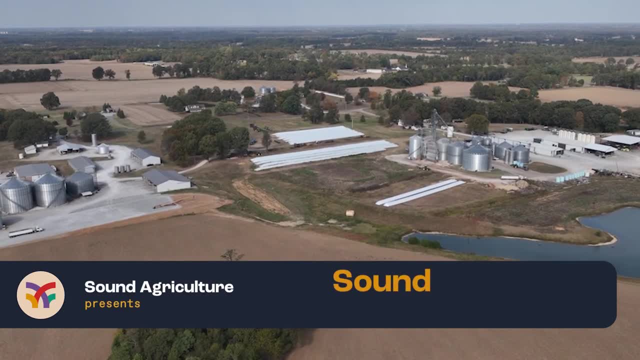 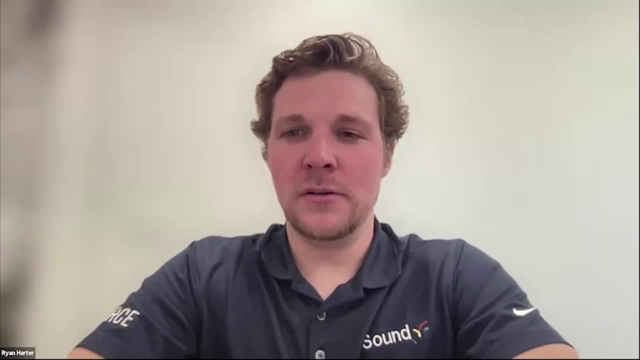 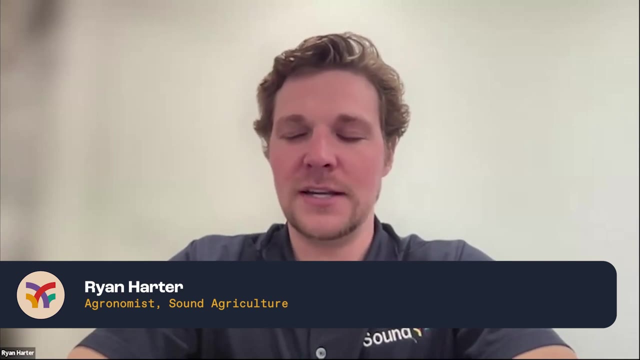 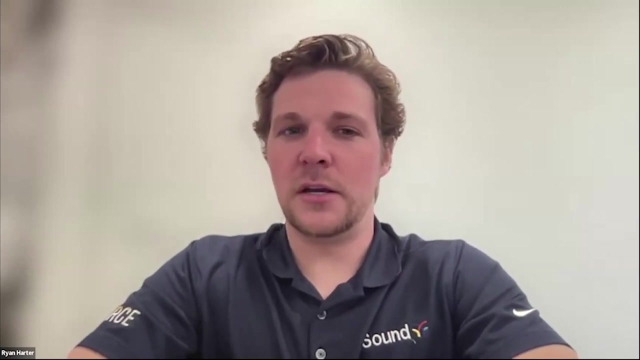 Hey everyone, Ryan Harder here, Technical Agronomist with Sound Agriculture in Missouri, Illinois and Wisconsin. In today's episode of Sound Advice we're going to be talking about Liebig's Law of the Minimum Mulder's Chart and how source can help on your acres. So stick around. 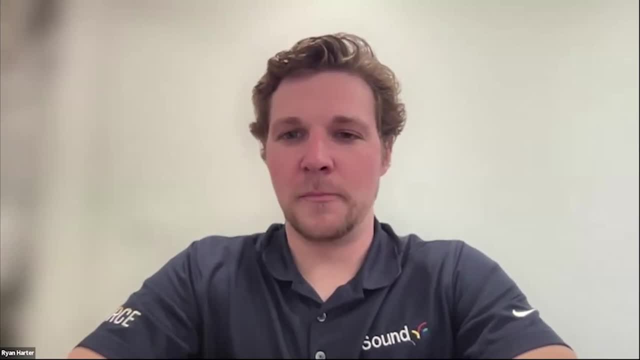 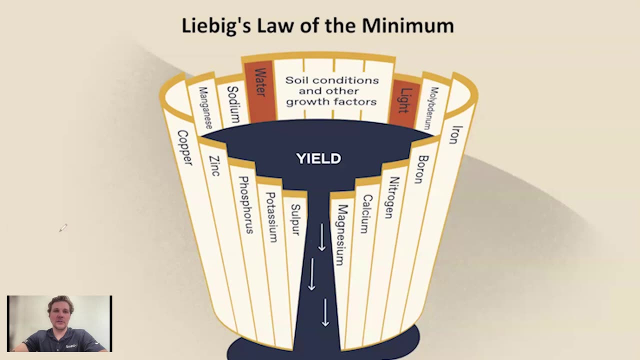 and see what we can learn about a new approach to fertility management on your farm. As we look at this graphic here that shows Liebig's Law of the Minimum, we can see that we have a barrel with different height of staves, And so when one stave is lower, 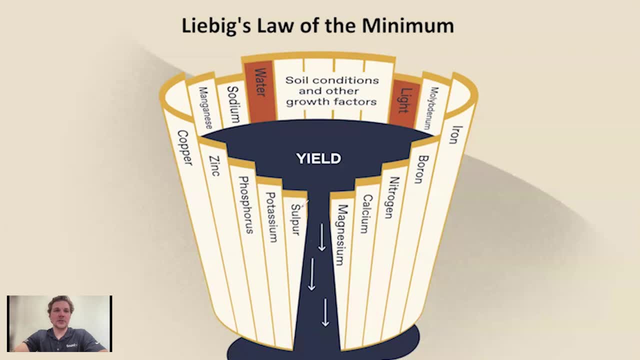 than another one. it's going to let the liquid inside out. So, in this instance, yield is the liquid that we're letting out. So when we have something that's limited, whether that be a micronutrient or macronutrient, it's going to limit the potential of the crop, Even though 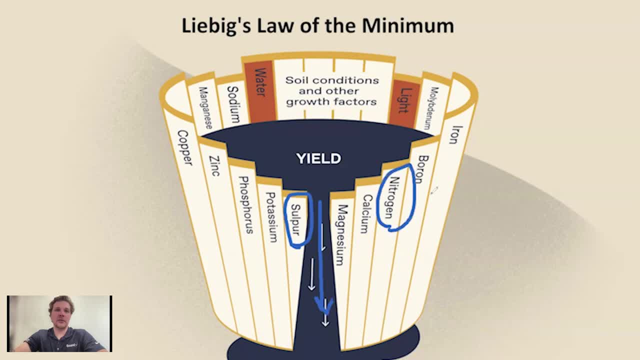 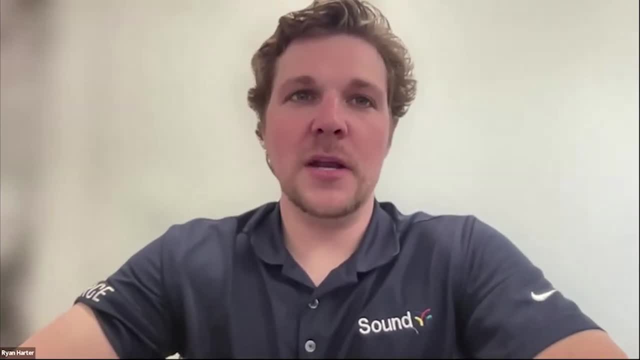 we might have several other factors that are in excess or in our favor of not limiting yield. any limiting factor is going to let our yield out. Now that we just learned about Liebig's Law of the Minimum, let's move on to Mulder's Chart And keep in mind what we learned on. 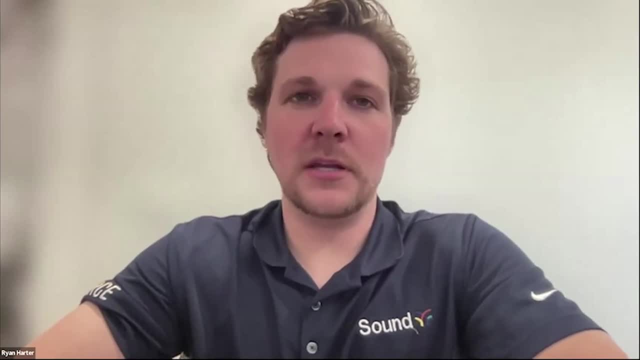 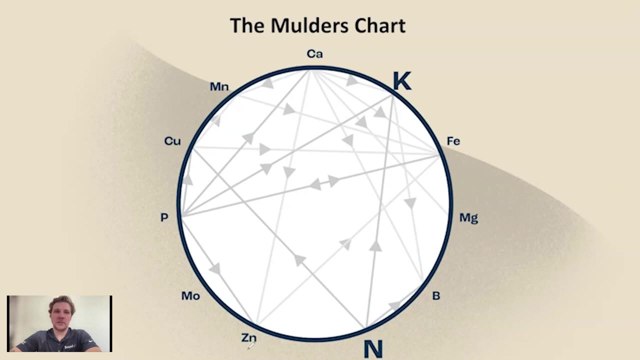 Liebig's Law of the Minimum and how that affects crop yield and your potential at the end of the year. As we look at Mulder's Chart here, we can see that we have arrows going in different directions with the nutrients on the outside, And so when we have an arrow going from one, 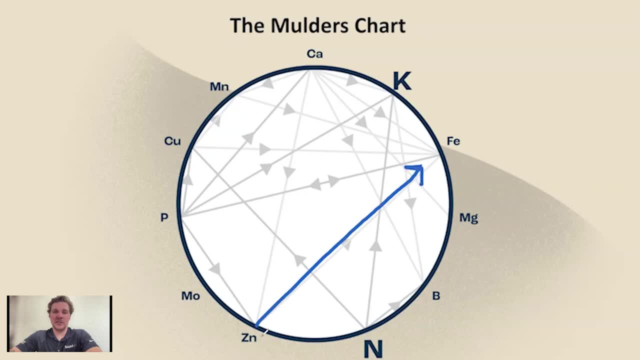 nutrient to the other. this shows us that when we have an excess of this nutrient, we're going to tie up the other nutrient, inducing a deficiency. So as we look at nitrogen and potassium, for instance, we can see that there's an arrow going from N to K. And so what that's? 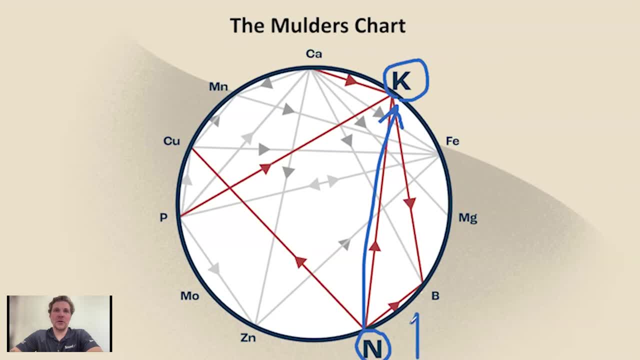 telling us is, when we over apply nitrogen and have an excess of it, we're going to limit the uptake that we have of potassium, therefore inducing a deficiency. So what does Mulder's Chart have to do with Liebig's Law? If we go back to the barrel, we might think that by 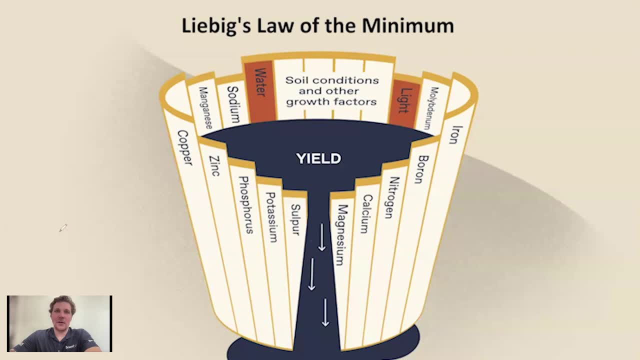 increasing nitrogen and making that stave higher, we're actually increasing our potential. But actually the opposite is happening. By making the stave on the nitrogen higher, we're actually shortening the stave on the potassium. So what we're doing by creating that potassium deficiency is decreasing potential yield. So the takeaway: